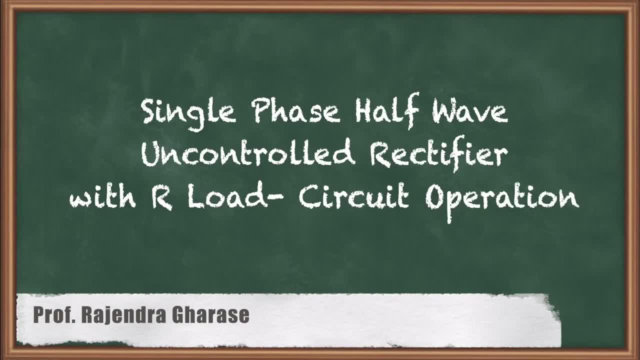 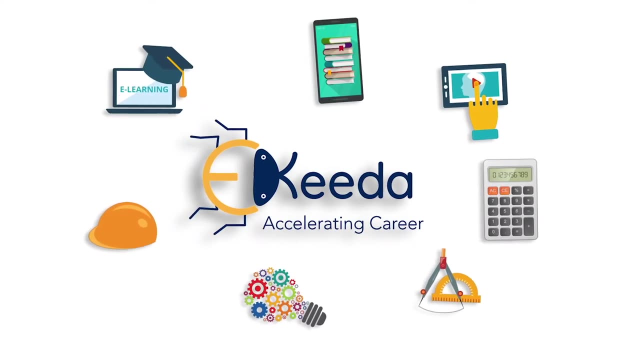 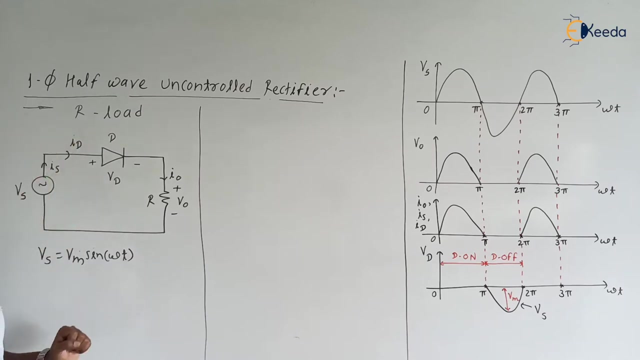 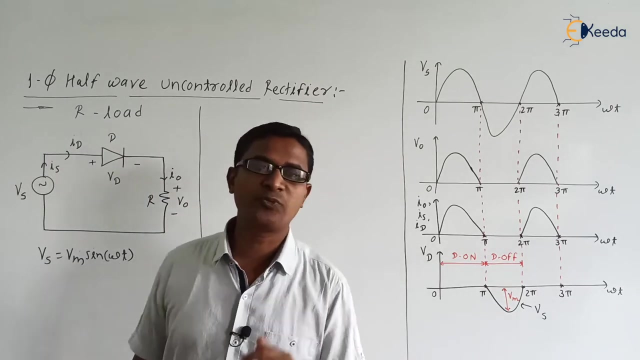 Hello friends, in this video we are going to discuss about the single phase half wave uncontrolled rectifier. Here it is the circuit diagram for single phase half wave uncontrolled rectifier with purely resistive load. So if you check the circuit diagram, as I said, the rectifier is the circuitry where input is AC and output is DC. 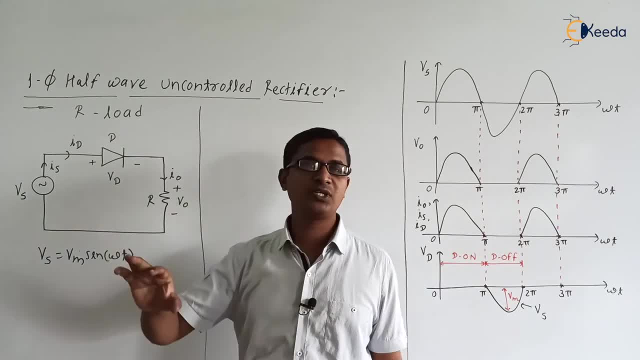 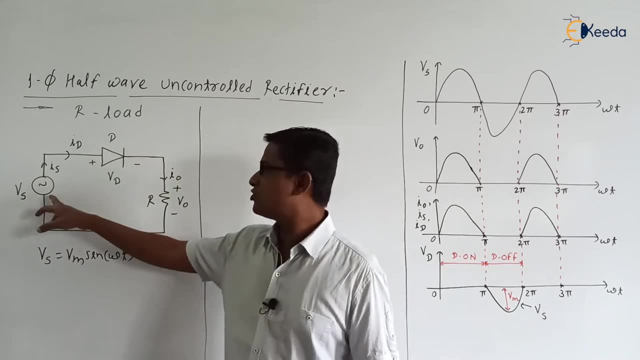 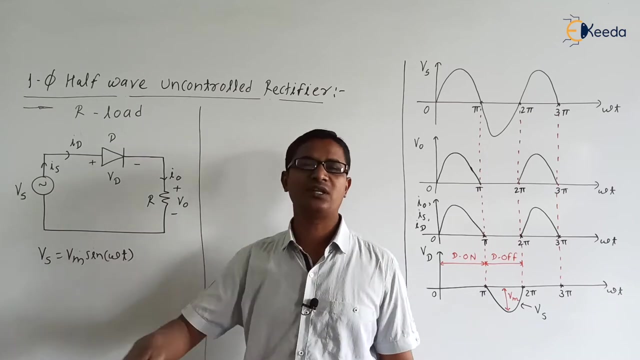 In the case of uncontrolled rectifier, the output is fixed DC. It is not the variable DC. Why it is fixed DC we are going to discuss. So the input is AC. So this is the supply. Vs is equal to Vm into sin of omega t, So it is a sinusoidal waveform. 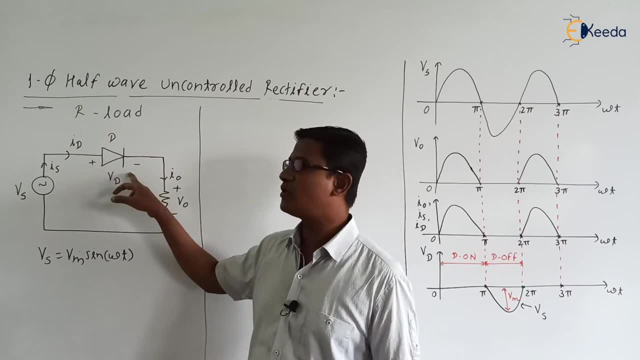 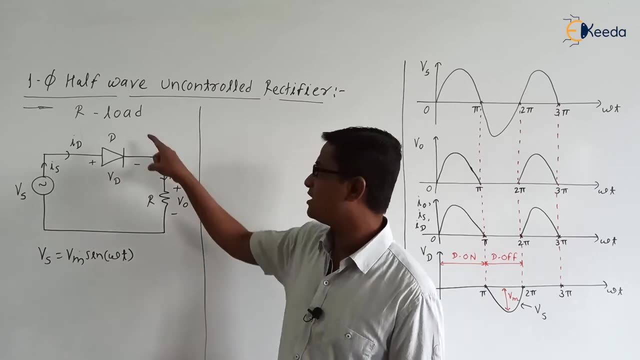 Next, here we are having the switch that is the diode. This is the uncontrolled switch, as this is the uncontrolled rectifier. So here we are having the switch is the uncontrolled switch. Next, as I said, the load is resistive. So here it is the supply switch and a load. 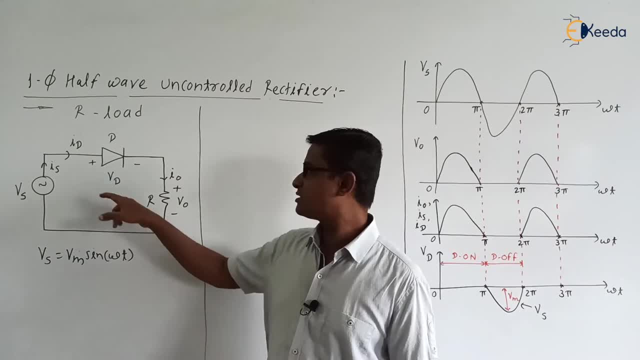 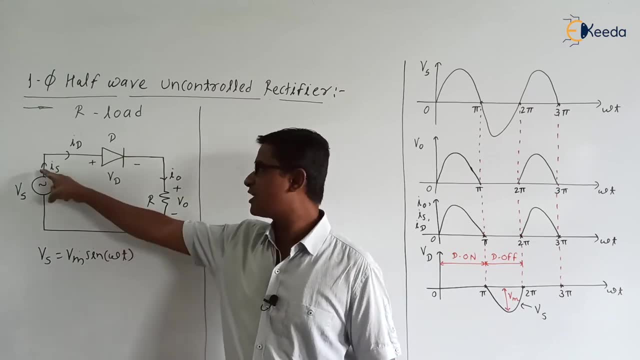 Supply switch and a load Next. the supply current is Is. Supply voltage is Vs. Supply current is said to be positive. if the direction of the Is is in the clockwise direction, Voltage across the diode is Vd. The Vd is said to be positive. 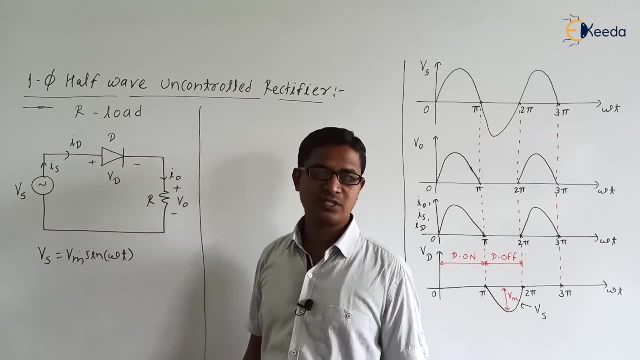 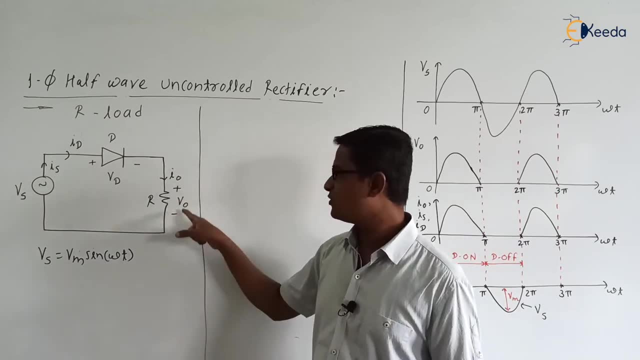 if here it is positive, Here it is a higher potential and here it is a lower potential, Otherwise it will be negative. Id is the current flowing through the diode. Voltage across the load is V0.. This V0 is said to be positive. if this potential is higher, this potential is lower. 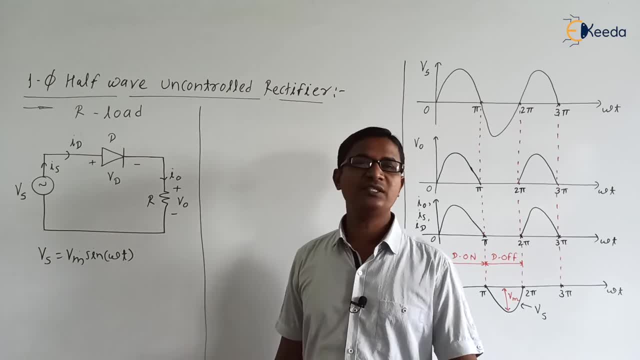 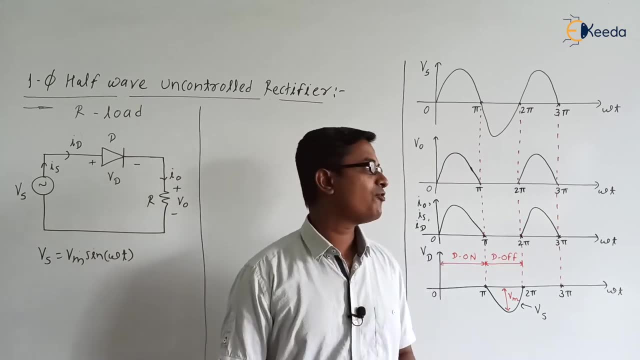 I0 is the current flowing through the load. The I0 is said to be positive if the direction of the current flowing through the load is in the downward direction. Next, in the waveforms, we are having the waveform of Vs, V0,, I0, Is, Id and Vd. 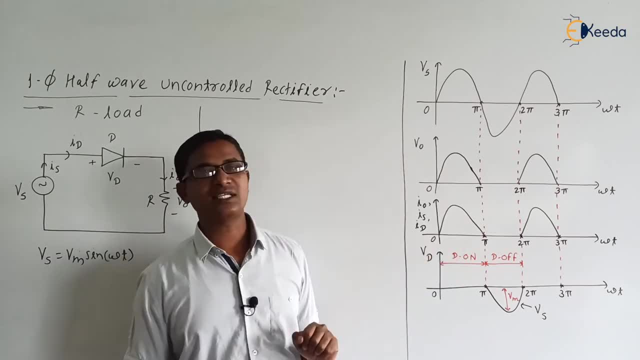 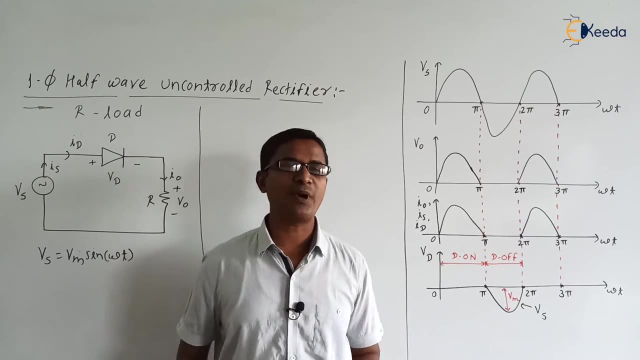 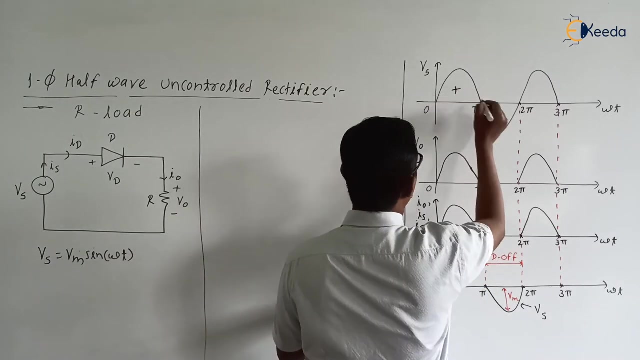 As I said, Vs is equal to Vm into sin of omega t. If you check from, omega t is equal to 0 to pi Vs is positive. From 0 to pi Vs is positive. From pi to 2 pi Vs is negative. 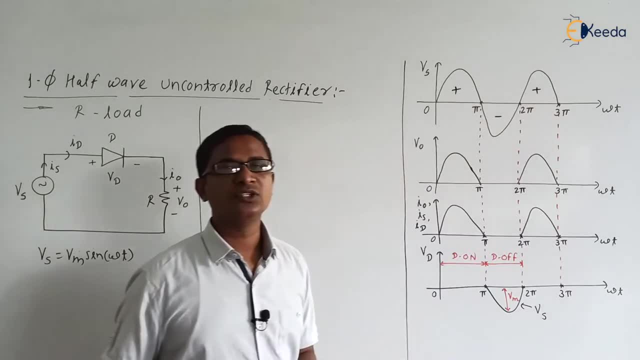 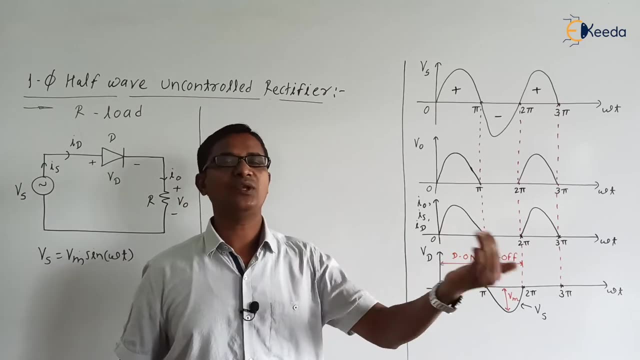 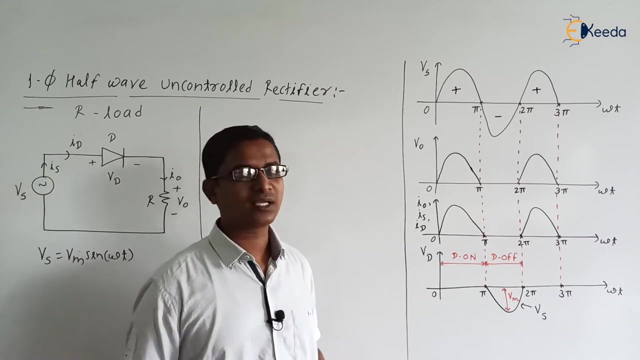 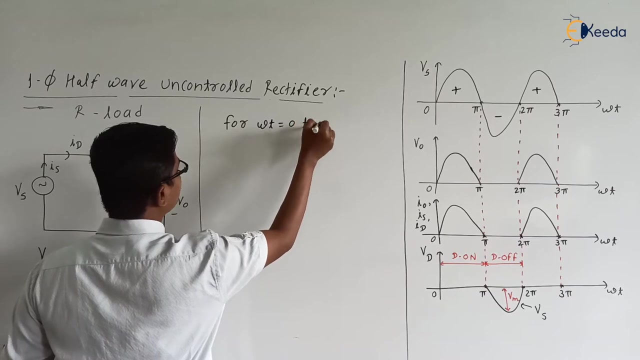 From 2 pi to 3 pi. it is positive In the supply voltage. we are having positive values, negative values, positive values and negative values Alternate. Now let us discuss the circuit operation. Suppose for omega t is equal to 0 to pi. 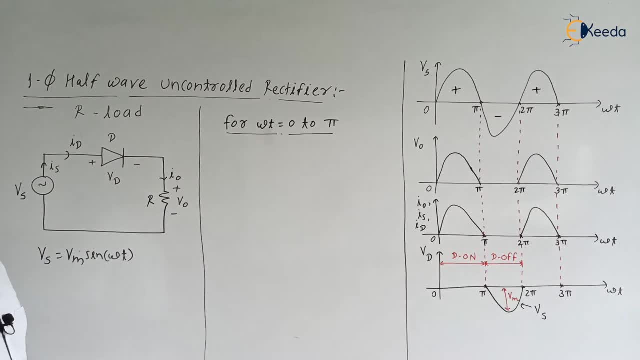 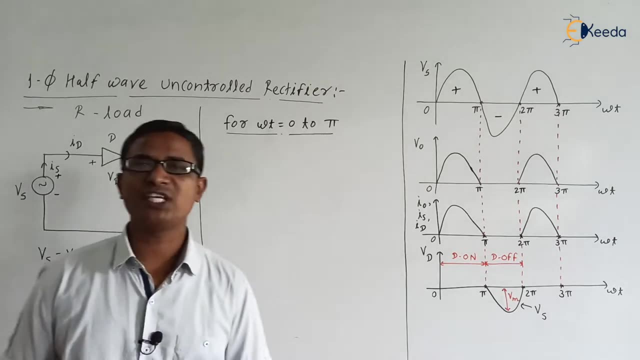 For omega t is equal to 0 to pi, Vs is positive. When Vs is positive, consider the polarities: plus here and minus here. For Vs positive if we consider: here it is plus, here it is minus. When Vs is negative it is positive. 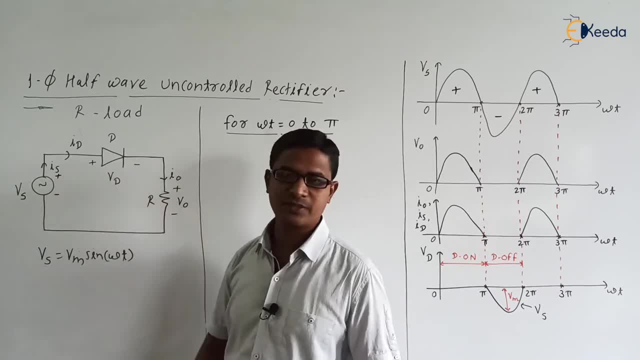 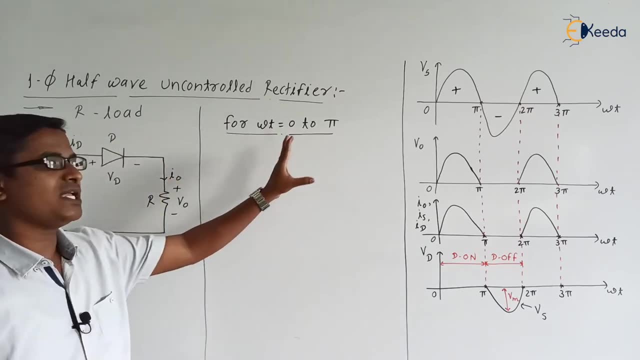 When Vs is negative, what will happen? This polarity should be reversed, Yes or no? Let us first discuss when Vs is positive, what will happen From 0 to pi? when Vs is positive, the polarity is plus here and here it is minus. 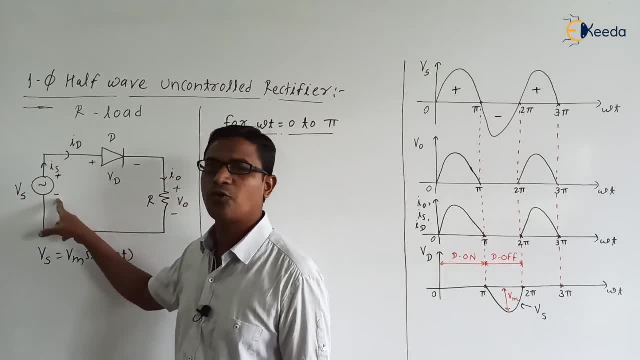 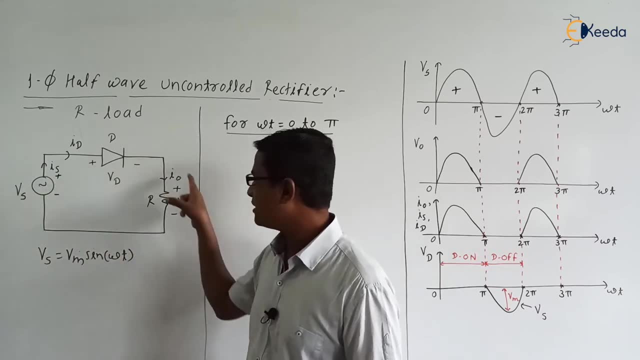 It is like this is the highest potential point in the circuit. This is the lowest potential point in the circuit. Highest potential is appearing at the anode of diode. Lowest potential is appearing at the cathode of diode. This is the highest potential. 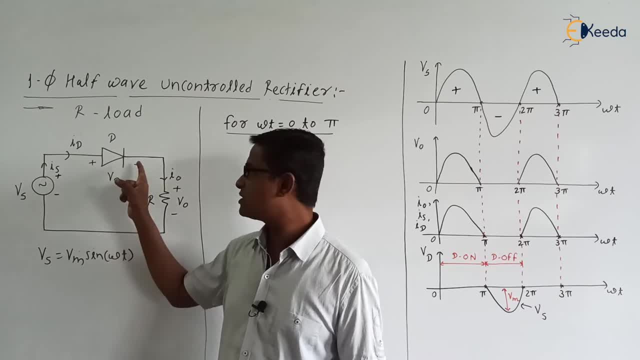 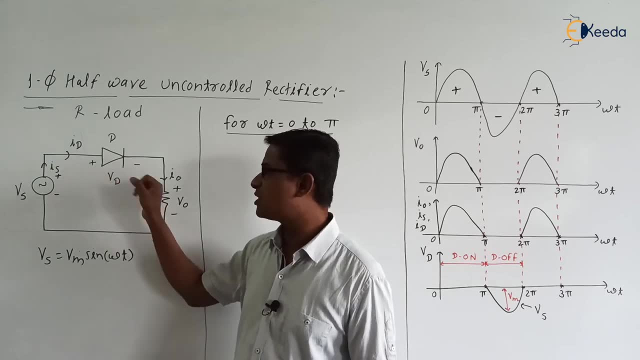 And the potential at the anode is the highest. So can we say that the cathode potential- definitely it will be lesser than that of the anode potential? Yes, So anode potential is higher than that of the cathode potential. 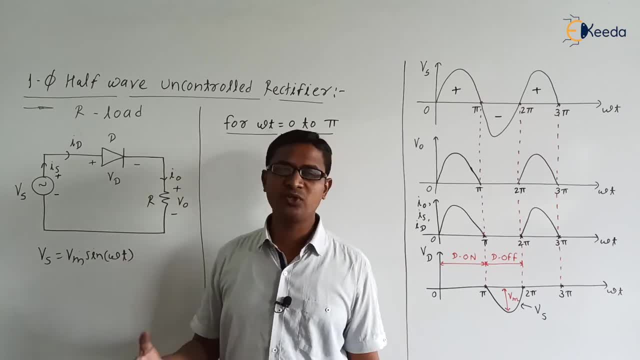 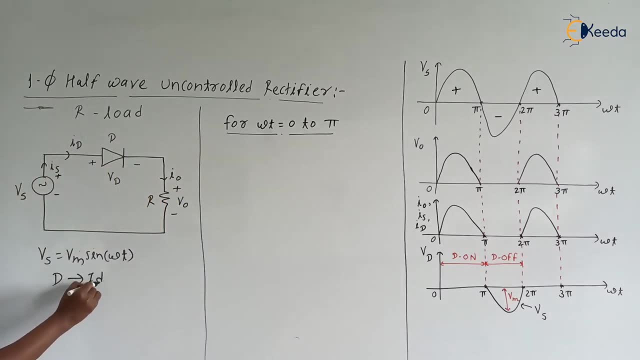 So can we say that the diode is in the forward bias mode? Yes, And as we know, suppose this diode is ideal diode. Suppose the diode is ideal diode. Diode D is an ideal diode. 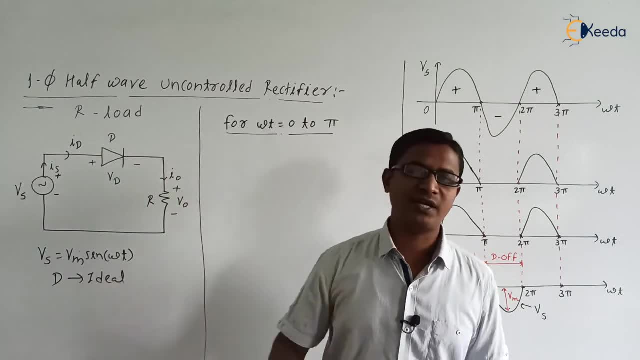 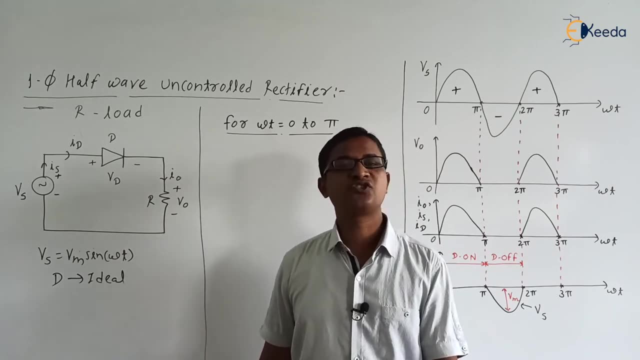 So, whatever the circuitry we are going to discuss in the rectifiers- Okay, In all the circuitries we are going to discuss we are going to consider the switch is nothing but the ideal switch. If it is a diode, it will be ideal diode. 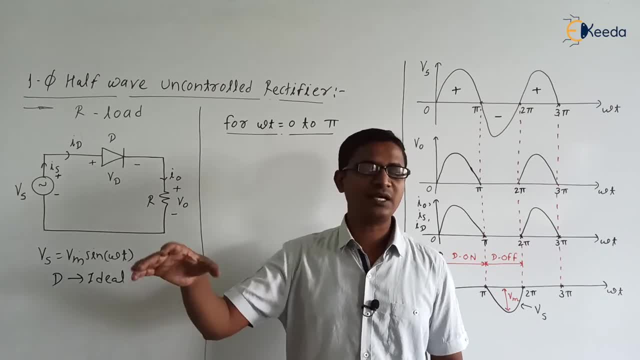 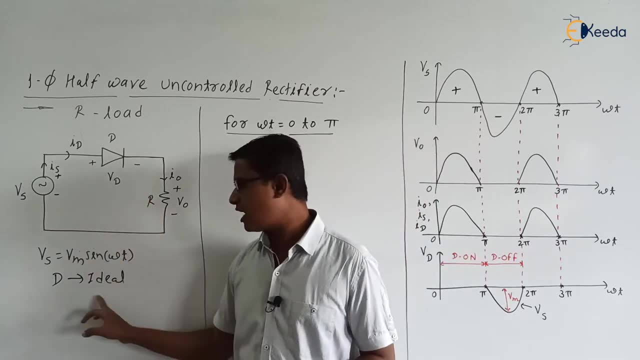 If it is a rectifier in the controlled rectifier, Okay. If it is a thyristor in the controlled rectifier, then we are going to consider it as an ideal thyristor, Okay, So next. So, here, as the diode is, ideal diode. 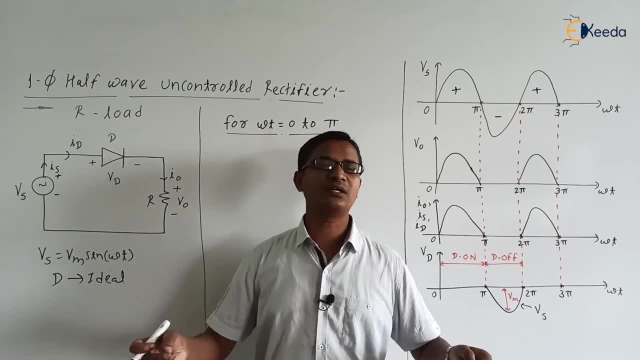 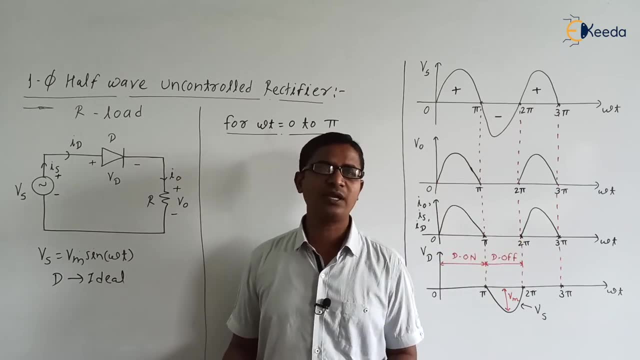 Okay, Ideal diode means what It is: the diode which requires a zero voltage Right, Or a very, very small voltage, 0.0000001.. It is approximately zero only. Okay To turn on. Are you getting the point? 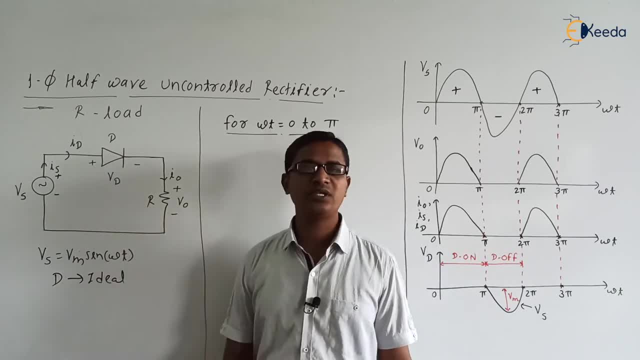 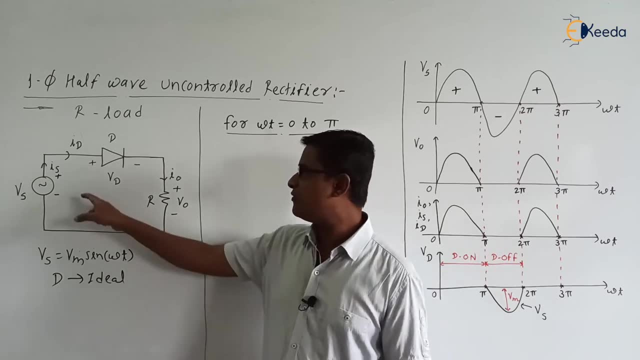 Okay So, and on state voltage drop of the diode: ideal diode is zero. On, state voltage drop of ideal diode is zero. Please note it. Okay Now. So when Vs is positive, highest potential is appearing at the anode of diode. 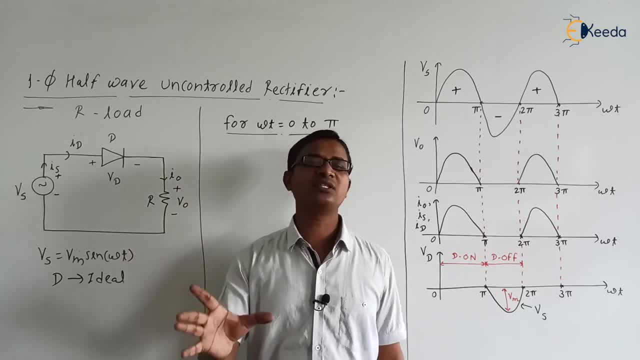 Lowest potential is appearing at the cathode of diode. So diode is in the forward bias mode And as the diode is in the forward bias mode, as we know, when diode is in the forward bias mode it turns on. 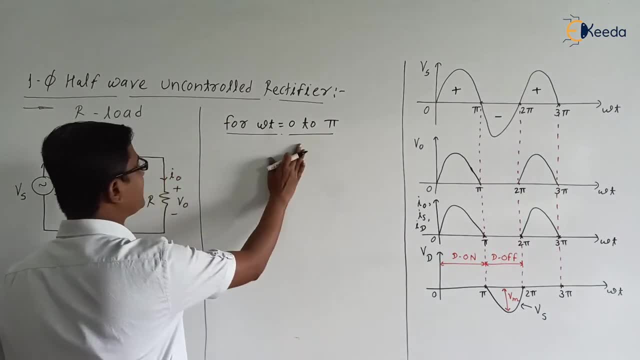 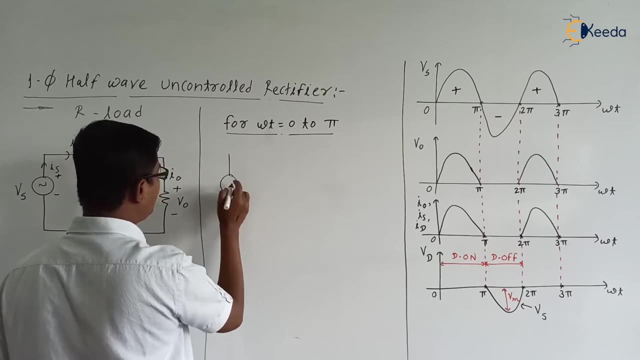 Are you getting the point? Okay, So here, from omega, t is equal to 0 to pi. Can we say that the diode is acting as a short circuit Means? it is in the on state. Okay, Diode is in the on state. 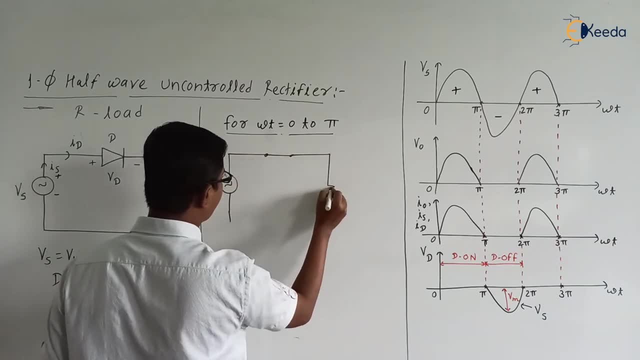 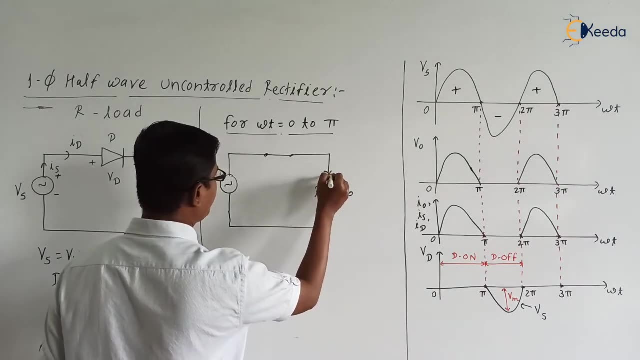 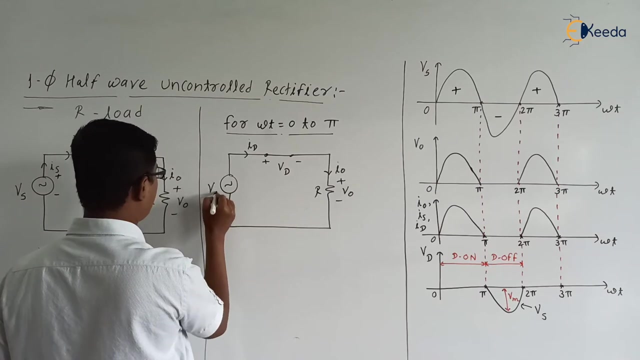 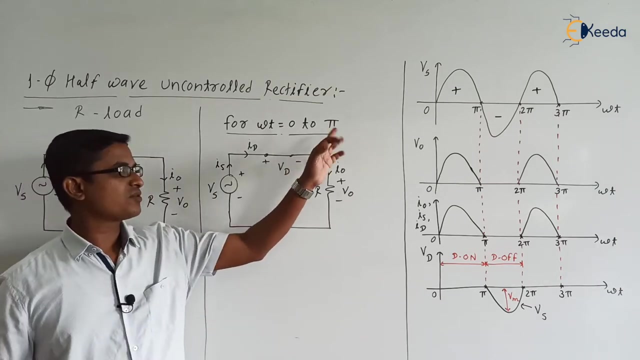 So we can draw the equivalent circuit like this. This is a resistor V0.. I0.. Vd. Id Vs Is Plus Minus, Right, So omega t is equal to 0 to pi Vs is positive. 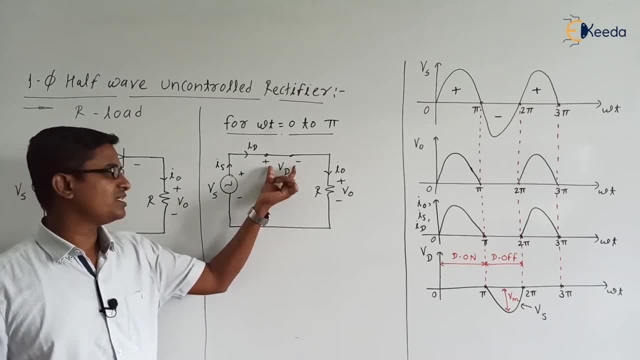 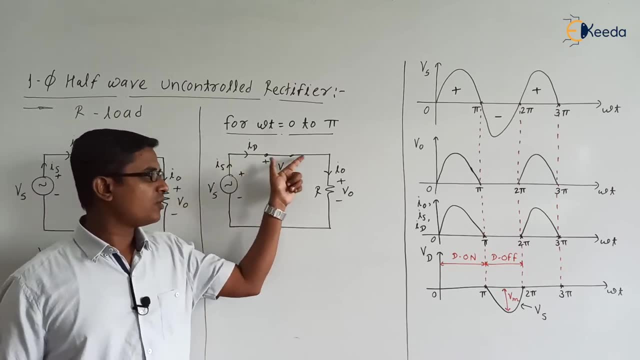 So plus here, Minus here. Diode is in the forward bias mode, So that's why it is acting as a short circuit. Okay, So in this circuit, if you check, yes, current will be flowing from Vs diode load and again back to the Vs. 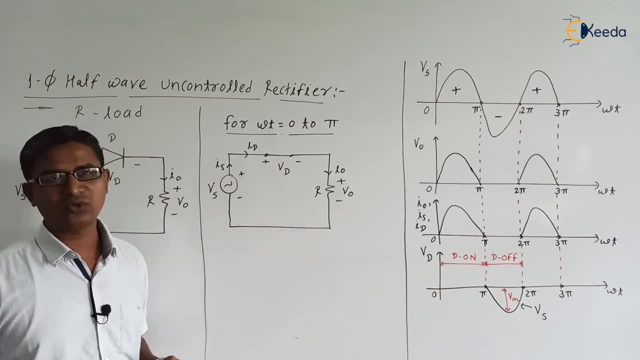 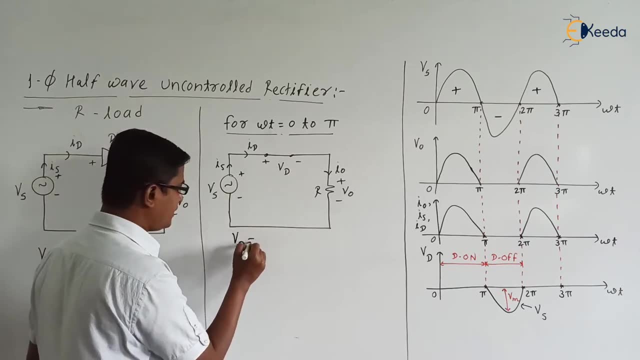 Okay, So current will be flowing in the clockwise direction, Yes or no? Okay, So now, what is the Vd Diode is acting as a short circuit. Okay, Vd is equal to 0.. Vd is equal to 0 volt. 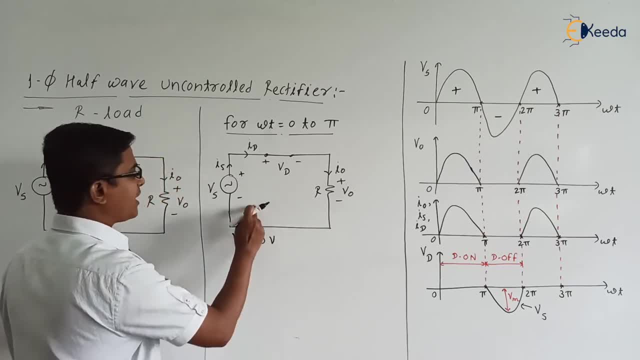 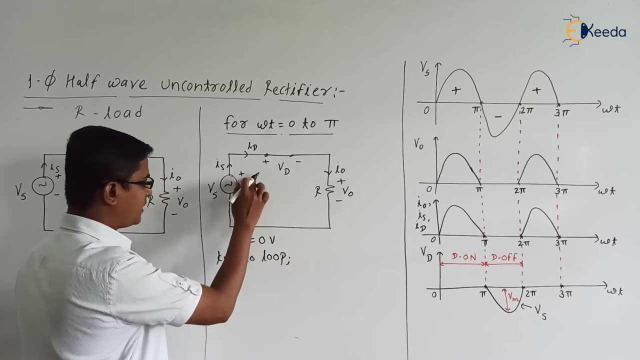 Are you getting the point Okay? Next, can we apply KVL to the loop? Yes, KVL to the loop. We can write it as KVL to loop. Yes, It is plus Vs minus Vd. minus V0 is equal to 0.. 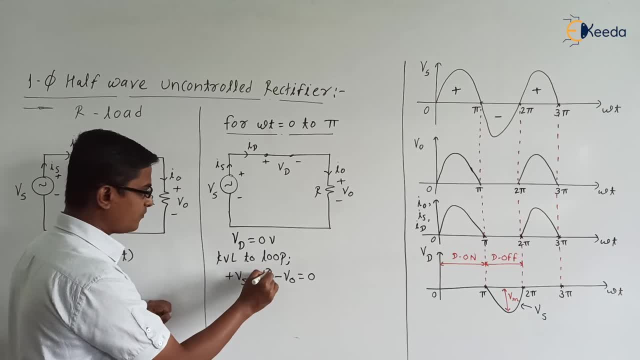 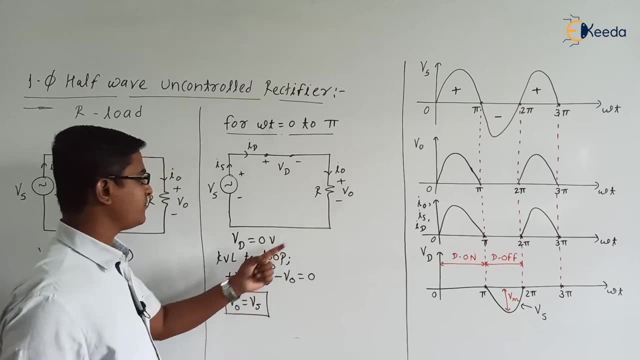 Right Again. what is Vd? Vd is 0. Right. So therefore can we write: V0 is equal to Vs. Very, very important. So load 1.. So load voltage is same as that of the supply voltage. 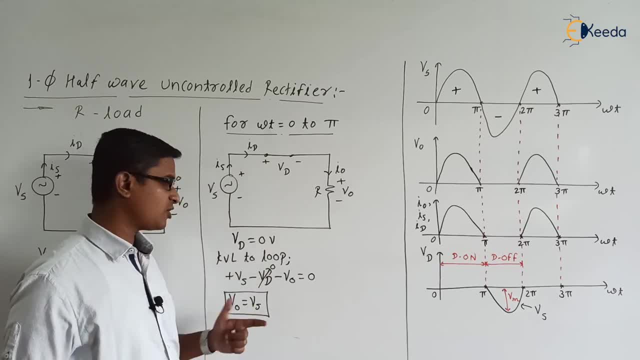 Okay, So from 0 to pi, load voltage is same as that of the supply voltage. Diode voltage is equal to 0.. Okay, Next, what is I0?? Can we write: according to the Ohm's law, V0 is equal to I0 into R? Yes, 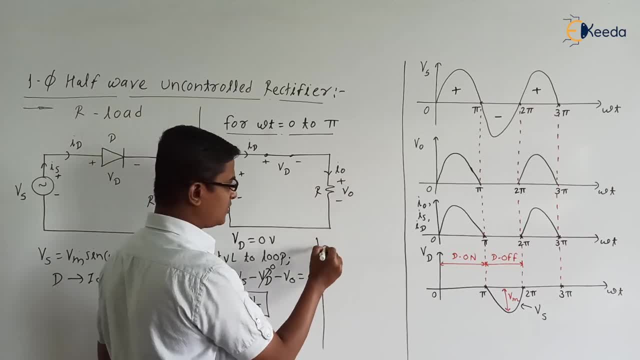 So therefore, I0 is equal to what V0 by R. Again, what is V0?? V0 is Vs, only Right, So we can write: I0 is equal to Vs by R. Okay, But we are having, yes, we are having- this circuitry. 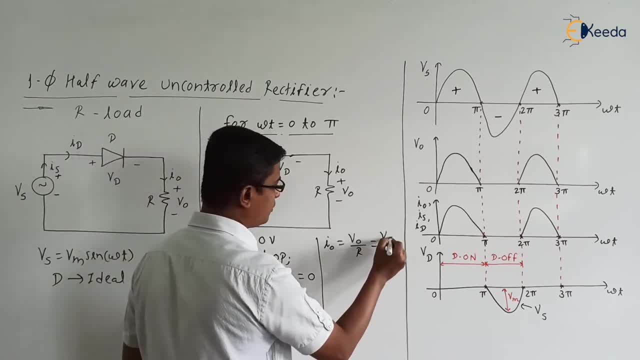 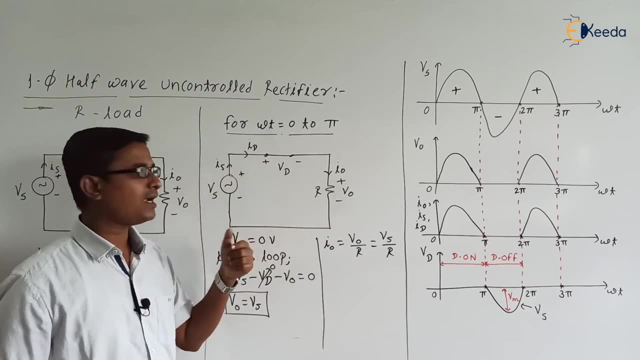 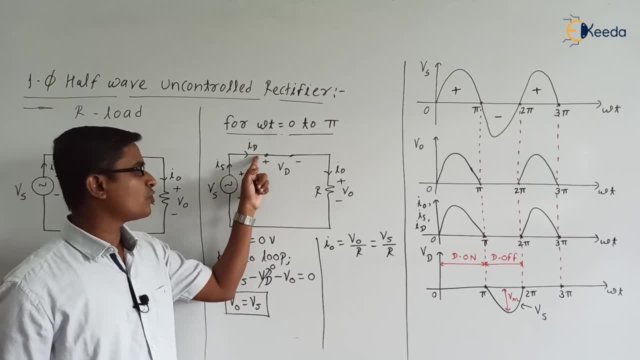 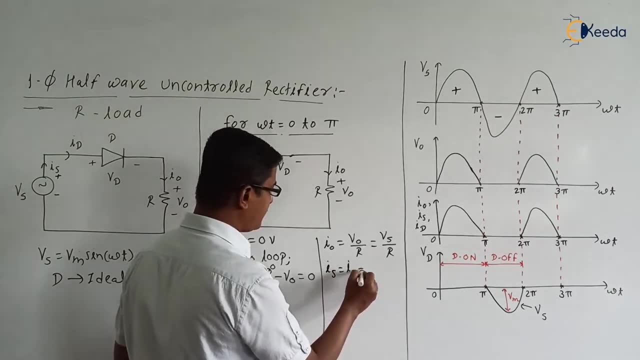 The same current will flow here. So can we say that Is is equal to Id, is equal to I0, is equal to Vs by R? Yes, So we can write it as: Is is equal to Id is equal to I0. is equal to what? 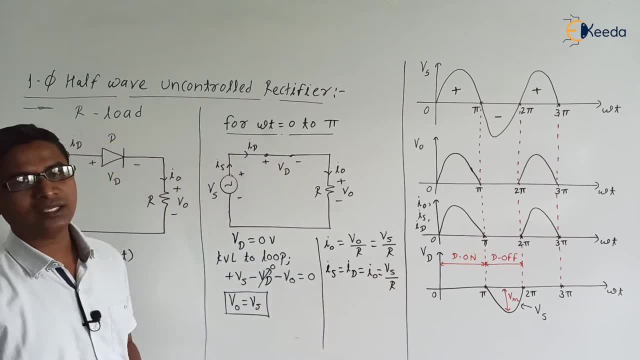 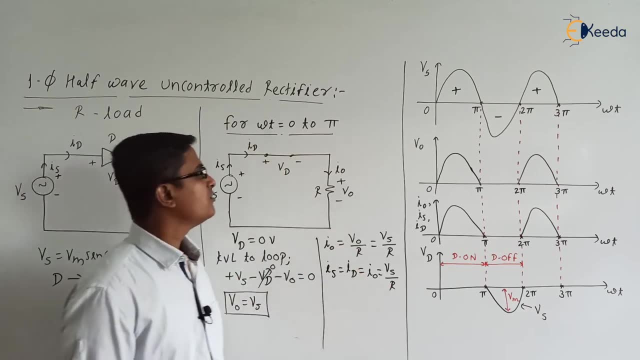 Vs by R. Are you getting the point? Okay, So this is for. omega t is equal to 0 to pi. Okay, Now from these values can we draw the waveform? Yes, omega t is equal to 0 to pi. vs positive we are having. okay, what is v 0? v 0 is same as that of 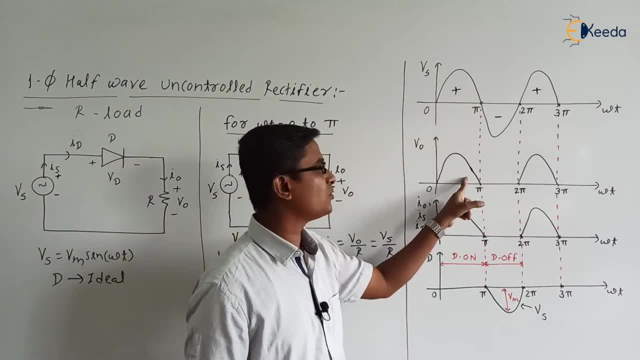 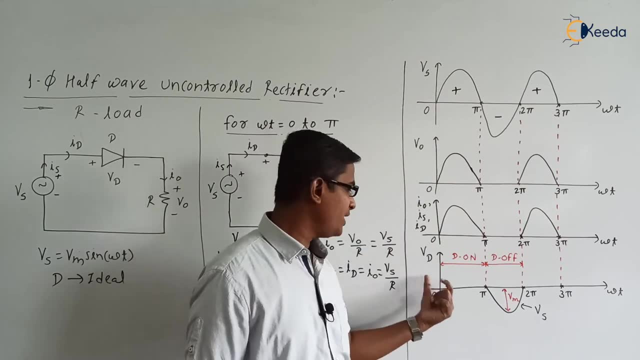 the supply voltage. okay, so v 0 will be same as that of the supply voltage. okay, so whatever the waveform for v supply voltage, the same will appear as a v 0, right? what is the vd? vd is equal to 0 because diode is in the on state. diode is acting as a short circuit. are you getting the point? okay? 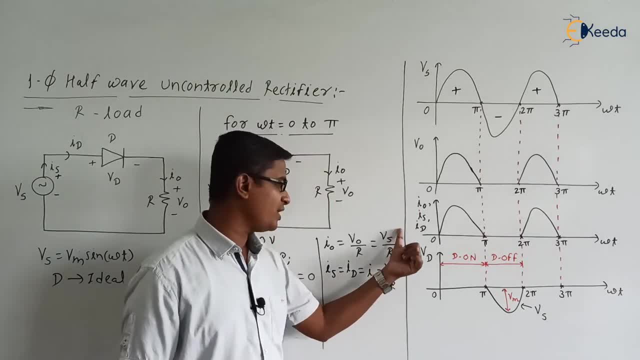 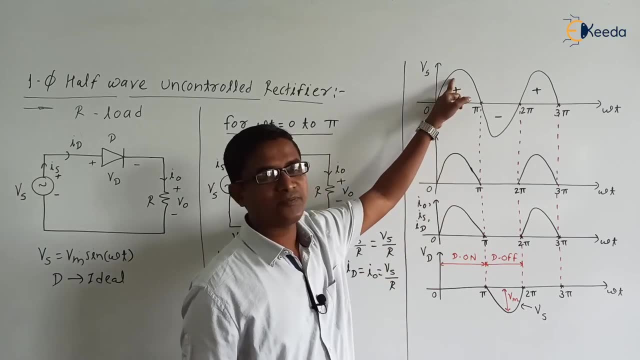 next, what is the i 0? yes, i 0 is equal to vs by r, and which is equal to id and is okay. so it is a vs by r. vs is vm into sine of omega t, okay, so definitely, yes, i 0 will be in phase with the v 0. 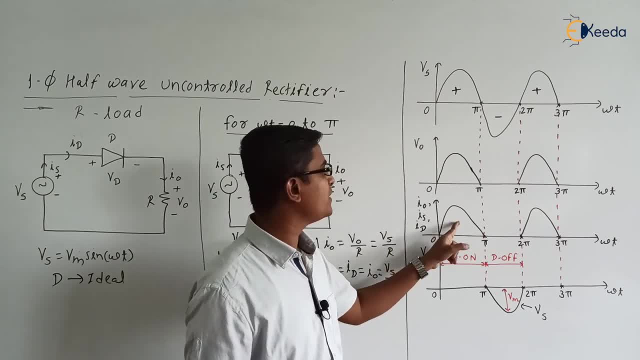 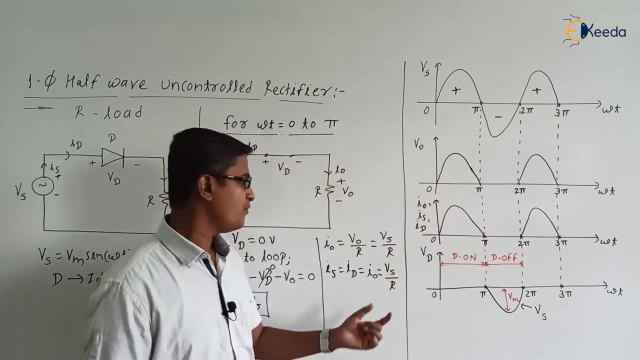 or the vs. are you getting the point? i 0 will be in phase with v 0 as well as vs. okay, if vs is maximum, v 0 will be maximum. so i 0 will be maximum because it is a vs by r or v 0 by r. are you getting? 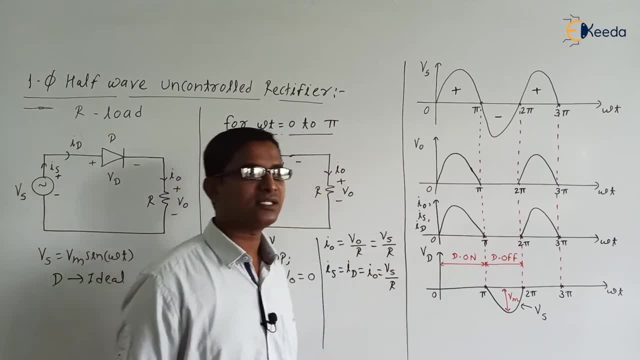 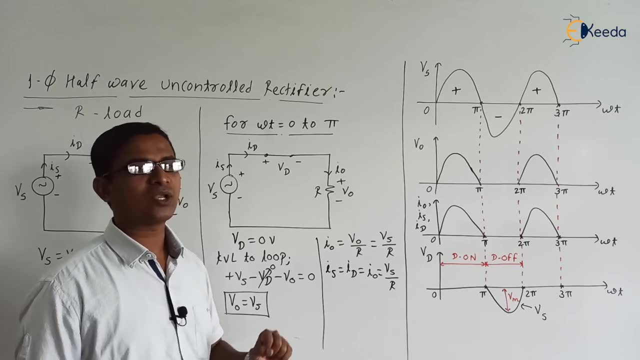 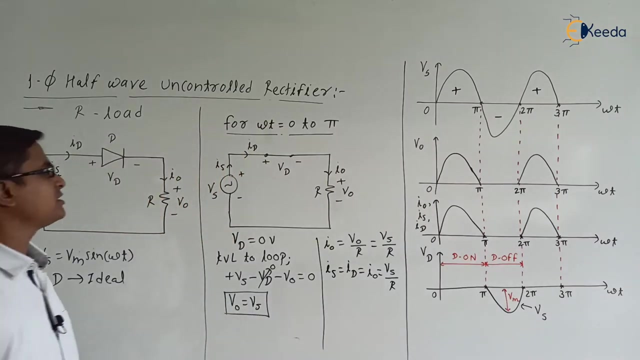 the point. okay, so this is the circuit analysis, for omega t is equal to 0 to pi. okay, now after pi, what will happen to the circuit we are going to discuss? okay, so if you check after pi, supply voltage is negative. okay, so here, from omega t is equal to pi to 2 pi. from omega t is equal to pi. 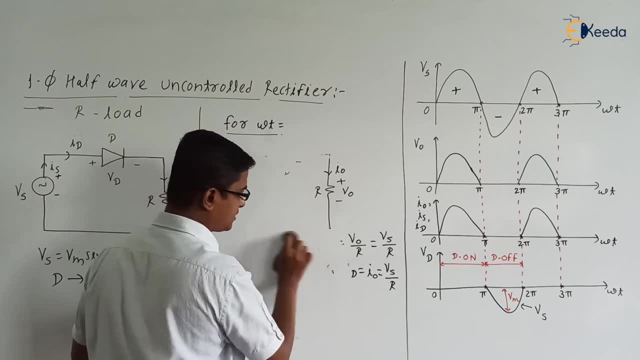 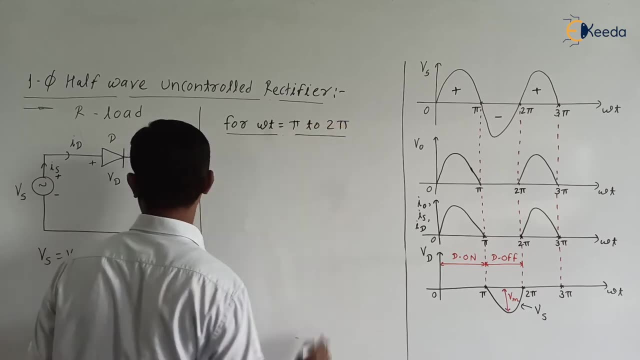 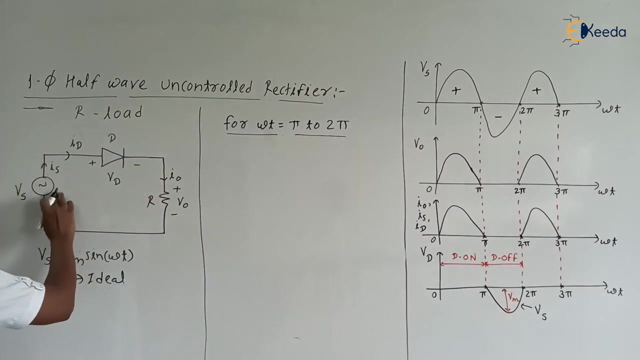 to 2 pi. let us discuss the circuit operation. omega t is equal to pi to 2 pi. okay, so yes, from pi to 2 pi, supply voltage is negative. okay, so, as supply voltage is negative, so we need to consider the polarity of the supply voltage. it has a minus here and here it is a plus. 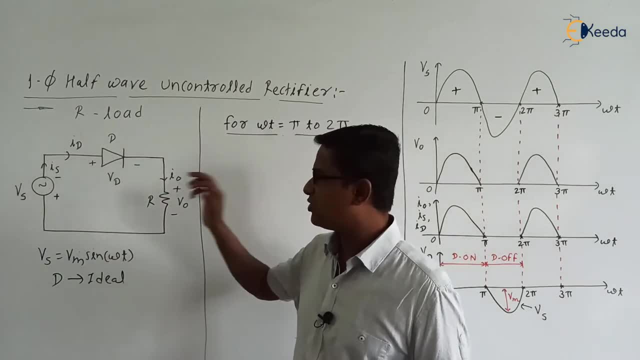 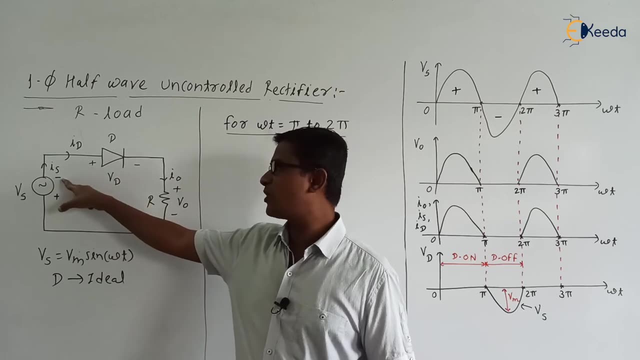 are you getting the point right? because supply voltage is negative. so i have reversed the supply voltage polarity. okay, so minus. here it is a plus here, so minus will appear at the lowest potential. here here it is the highest potential, so lowest potential is appearing at the anode of diode. 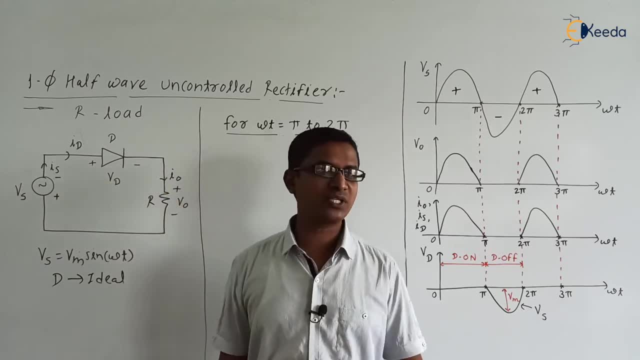 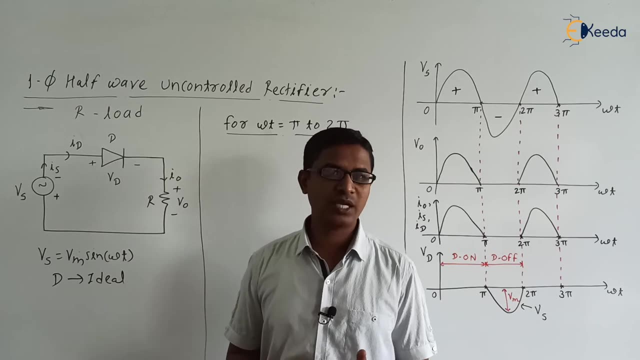 highest potential is appearing at the cathode of diode. okay, so can we say that when vs is negative, that is from omega t is equal to pi to 2 pi, diode will fill the reverse voltage. okay, and when the diode is in the reverse bias mode, what will happen? diode will act as an open circuit. 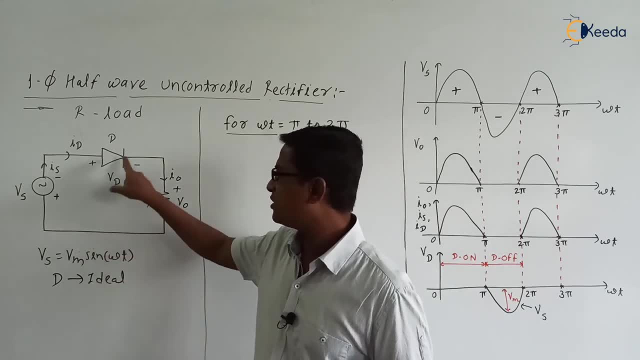 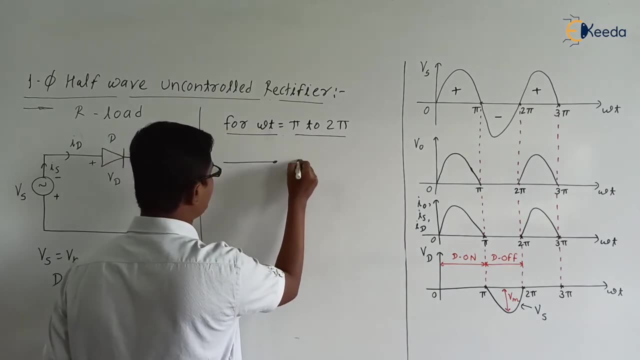 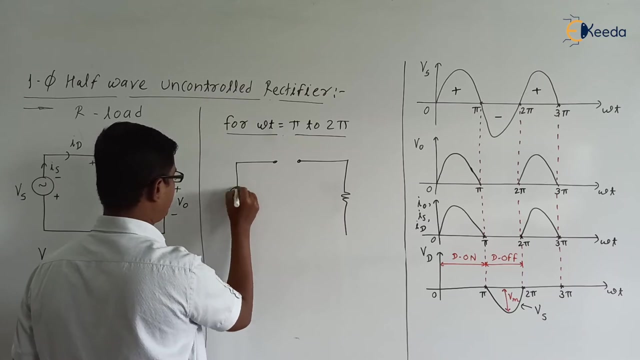 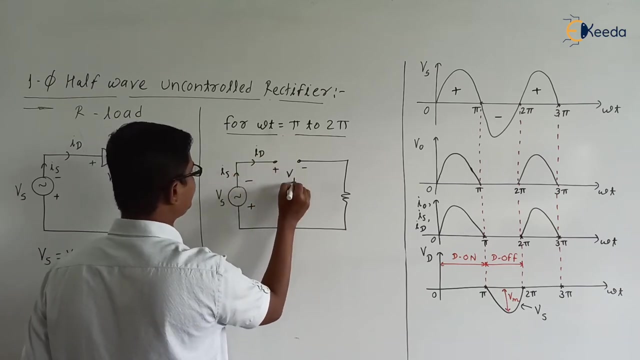 okay, are you getting the point? okay? so when vs is negative, this diode will act as an open circuit, okay, or it will act as an off switch. okay, it will act as an off switch. yes, this is a vs minus plus. this current is id. this one is: is this voltage is vd, this is i0, this is resistance, this is a v0. 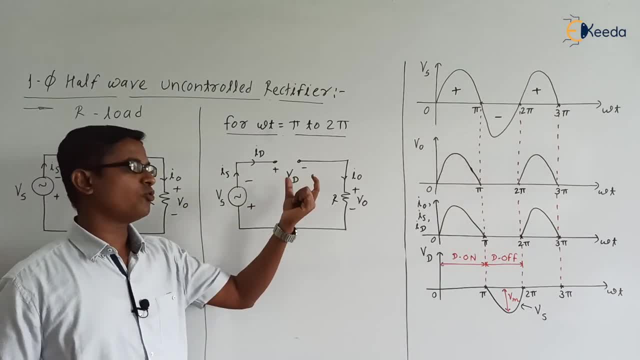 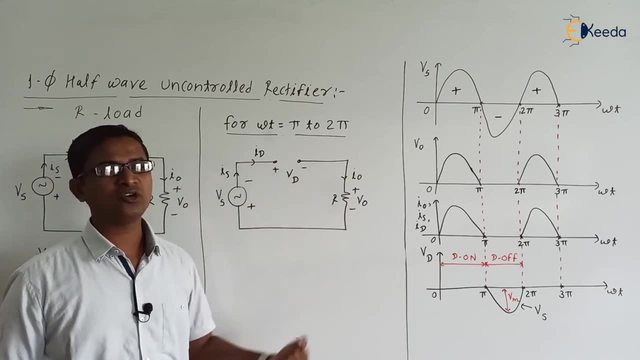 okay now. so from pi to 2 pi diode will act as an open circuit. okay means it will act as an off switch. okay. so now when the diode is in the open circuit mode? when the diode is in the open circuit mode, what about the current in the circuit? in the current in open circuit is always. 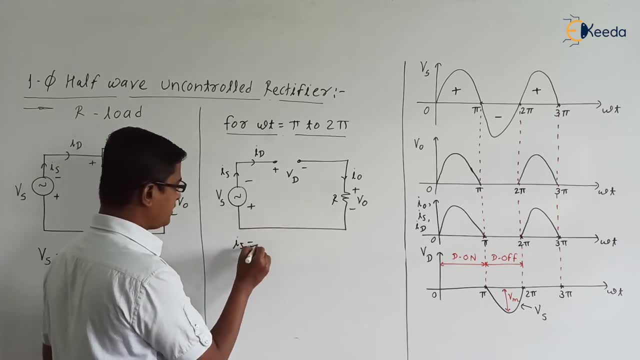 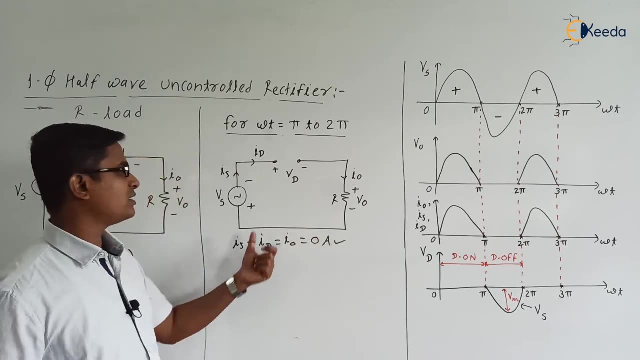 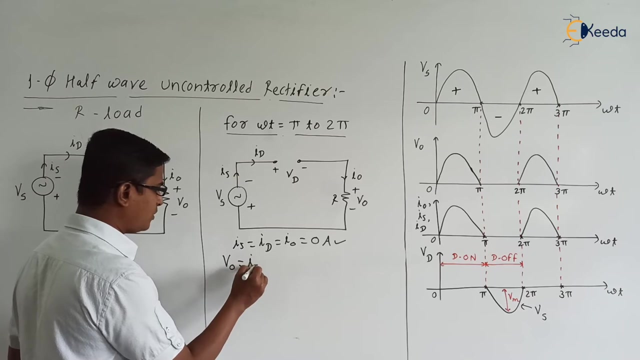 zero. okay, so can we write it as is? is equal to id, is equal to i0. is equal to what zero ampere? are you getting the point? okay, so currents are zero ampere, okay. next, if current is zero ampere, what is the v0? according to ohm's law, v0 is equal to i0 into r, so is equal to zero volt. 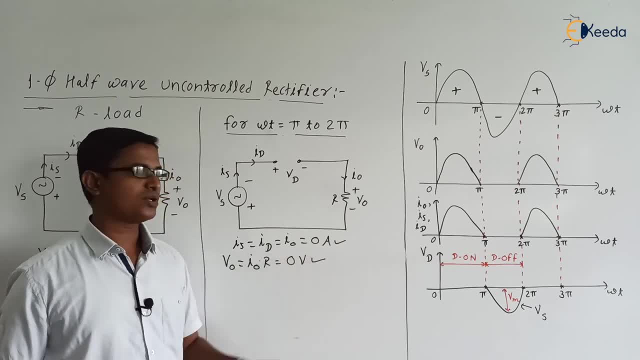 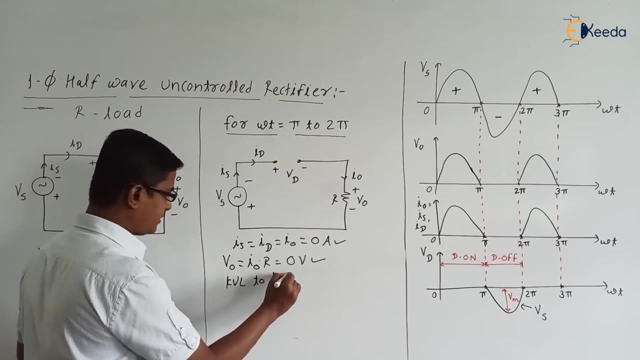 are you getting the point? so v0 is zero, i0 is also equal to zero. can we apply kvl to the loop? yes, we can write kvl to loop. yes, it is minus vs minus. vd minus v0 is equal to zero. but what is v0? v0 is zero because we are. 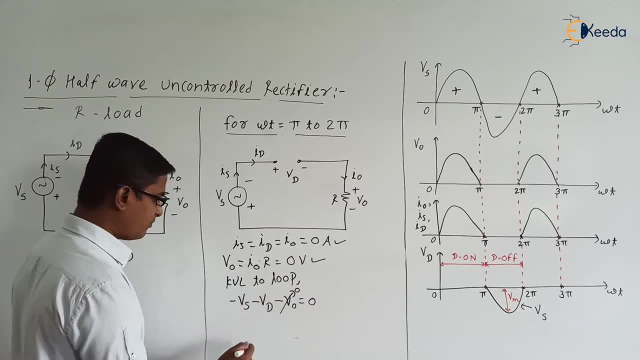 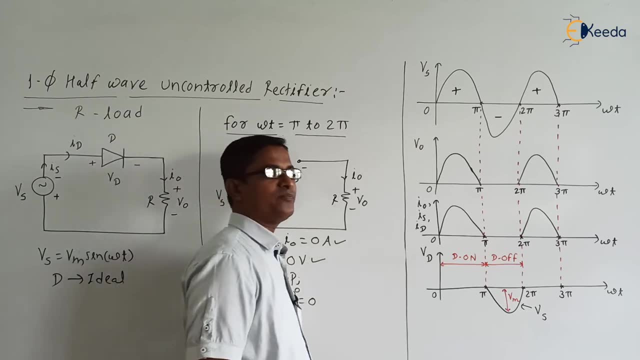 having v0 is zero, okay. so from this can we write: vd is equal to minus vs. yes, vd is equal to minus vs means the voltage across thyristor- sorry, voltage across diode is equal to minus vs. right voltage across diode is equal to minus vs. okay. so if you check the circuit, you will get the 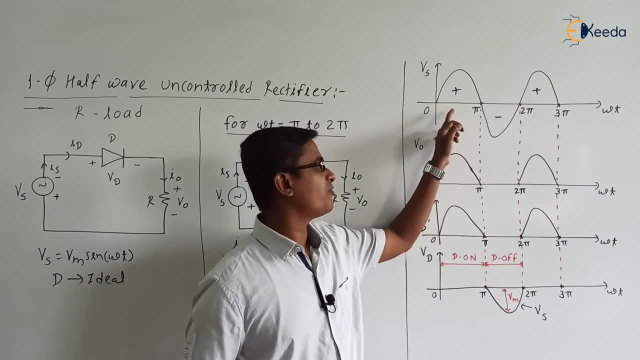 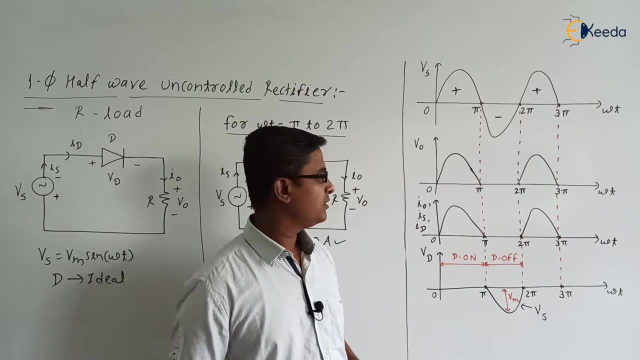 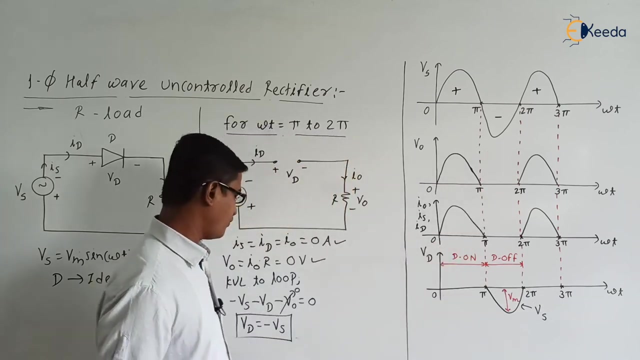 circuit from omega t. sorry, if you check, the waveform from omega t is equal to pi to 2 pi right from pi to 2 pi. v0 is zero, right. i0 is zero, right. and what is vd? vd is negative, but it is same as that of the supply voltage, right? so vd is negative, but it is the same as that of the. 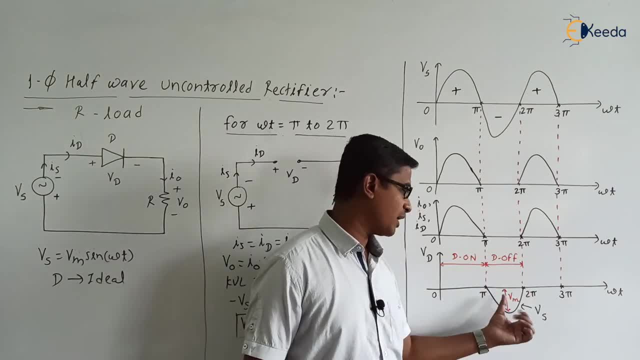 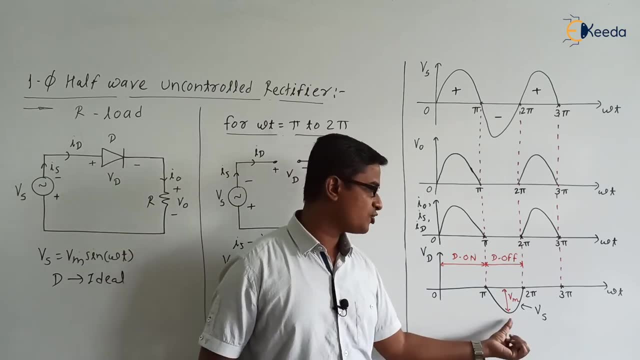 supply voltage, so negative voltage will appear across the diode. okay, because the supply voltage is negative, so diode is in the reverse bias mode. so that's why the voltage across the diode should be negative. are you getting the point? okay, so whatever the pulse here, the same pulse. 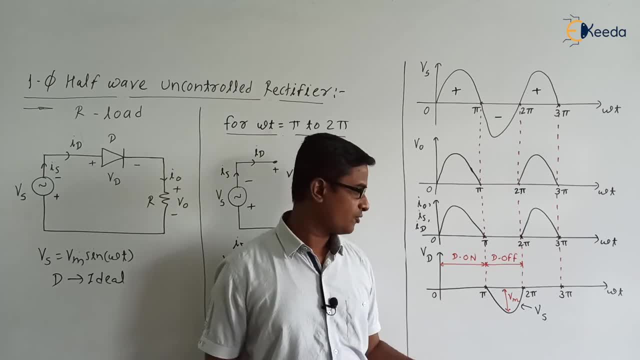 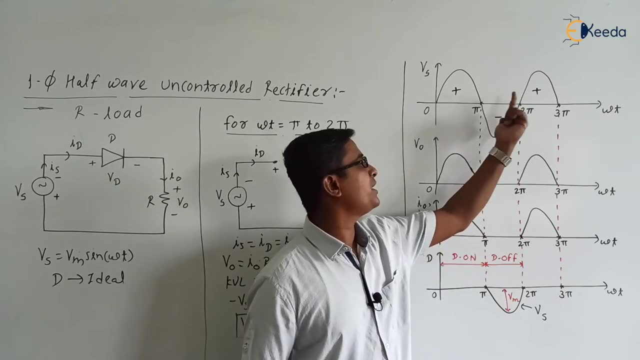 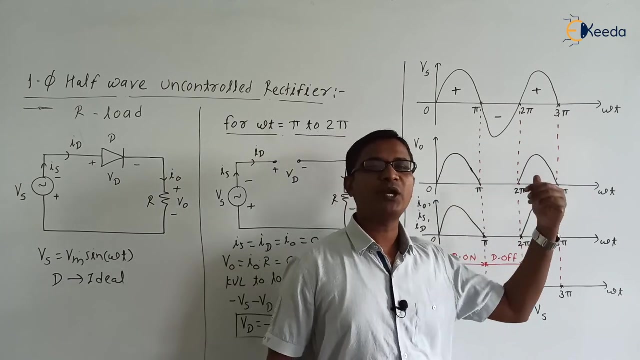 will appear as a reverse voltage for the diode. okay, so, from pi to 2 pi, diode is in the off state. similarly, after 2 pi, what will happen? yes, after 2 pi, the same cycle is repeating. okay, so, whatever the output we are having, from 0 to 2 pi, the same goes on repeating. from 2 pi to 4 pi, 4 pi to 6 pi. 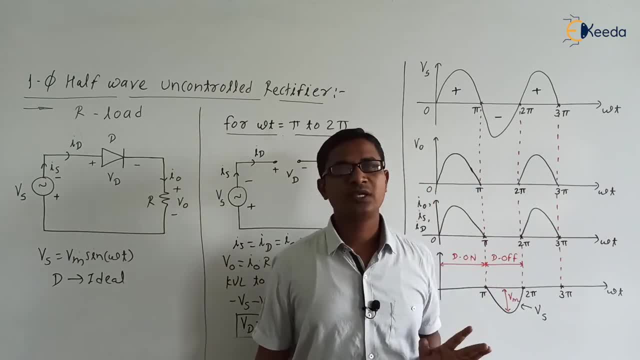 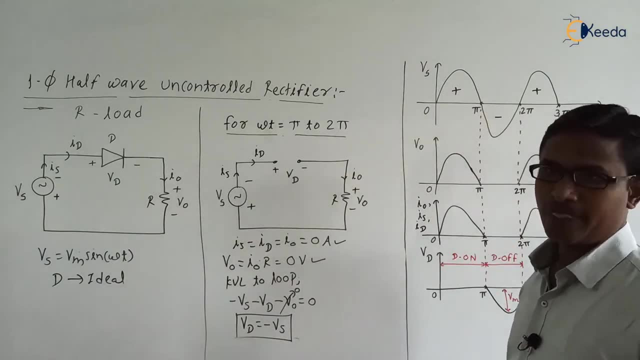 and so on. are you getting the point? okay? so here why it is known as the uncontrolled rectifier. if you check, yes, corresponding to one input cycle in the output, we are getting one positive half cycle only in the output. we are getting the positive half cycle only, okay, corresponding. 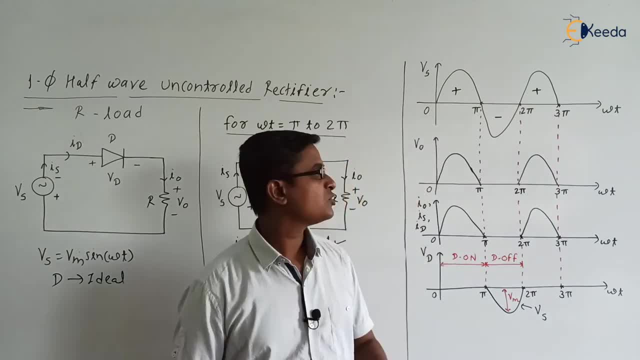 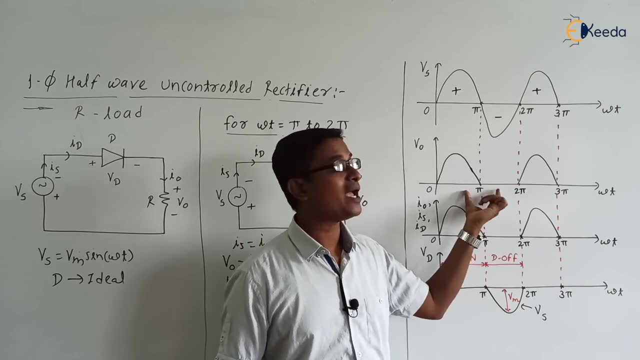 to the negative half cycle in the output, we are getting the zero voltage okay. so that's why it is known as the single phase half wave rectifier. single phase half wave rectifier. are you getting the point? why halfway? because we are rectifying only half wave corresponding. 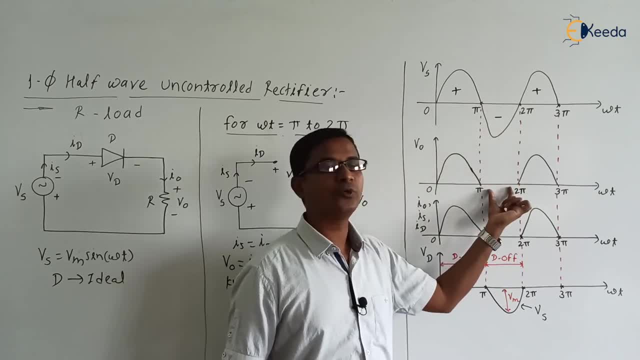 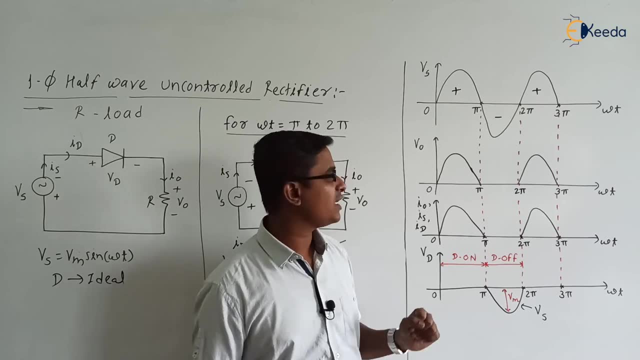 to the second half wave. that is a negative cycle. we are getting the zero output. so that's why it is a single phase half wave rectifier. okay, now in the output. if you check in the output, yes, can we vary this output? no, because diode is the uncontrolled switch and after omega t is equal to. 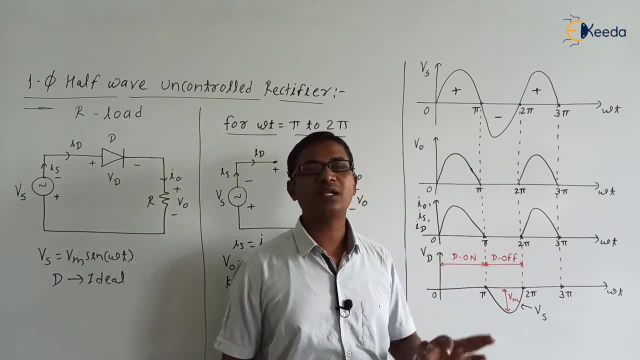 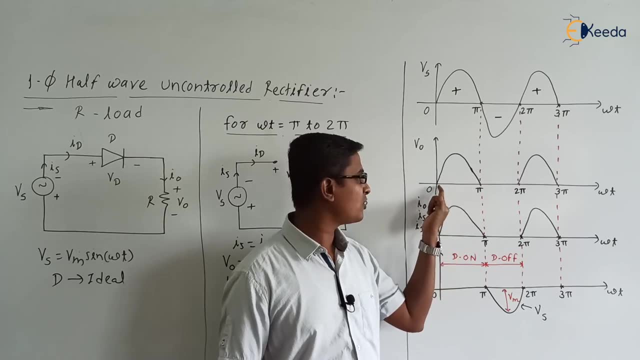 zero, the diode automatically turns on. okay means here we cannot turn on the diode at this instant. or at this instant or at this instant: okay, diode will automatically turn on at this instant, only that is, at omega t is equal to zero. only okay means in the output. okay, we will be getting. yes. 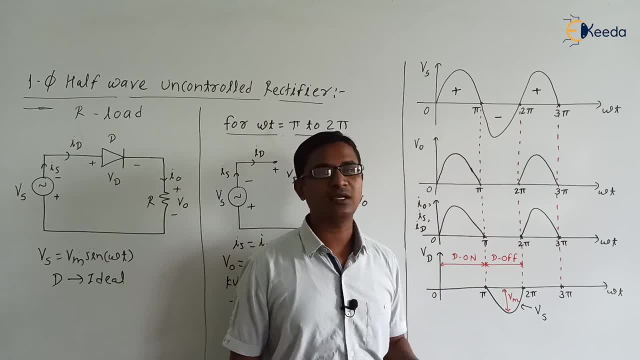 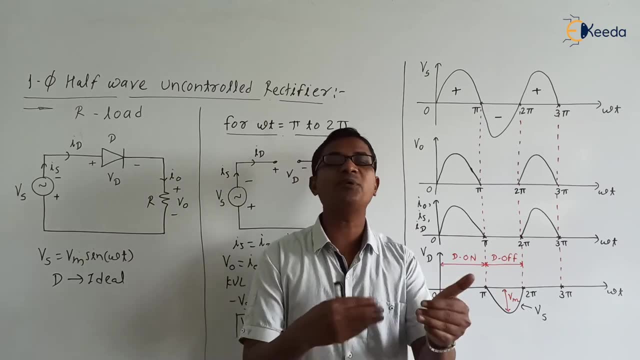 half cycle. full half cycle, that is a full, positive half cycle of the supply. are you getting the point? okay, that's why it is the uncontrolled rectifier. okay, means output voltage cannot be varied. output voltage cannot be varied. are you getting the point? okay, if we are having the fixed, 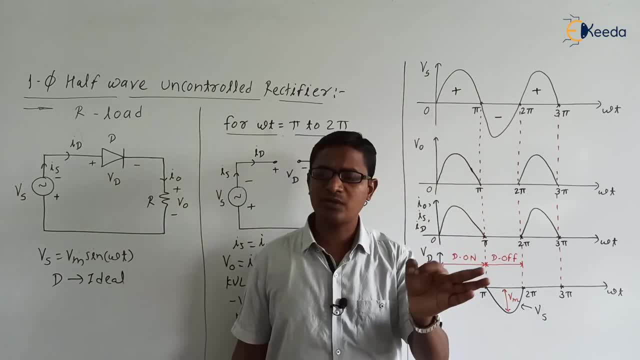 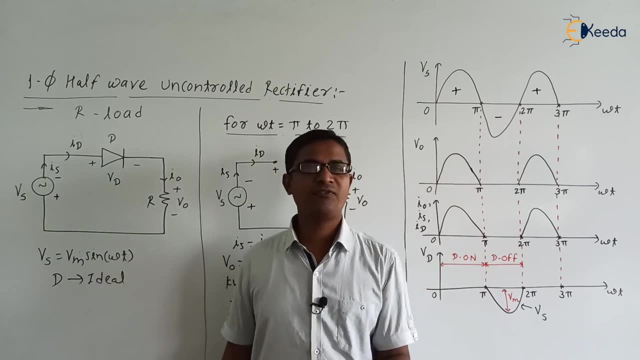 input voltage, then output voltage. whatever the output voltage will be getting is constant. only are you getting the point, okay? so that's why it is known as the single phase half wave uncontrolled rectifier. next, corresponding to one input cycle. in the output, we are getting only one pulse. okay, corresponding to: 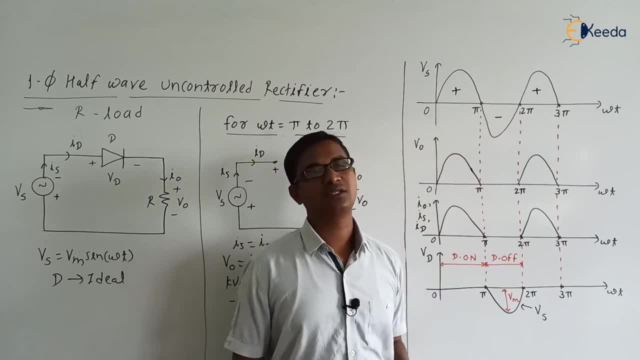 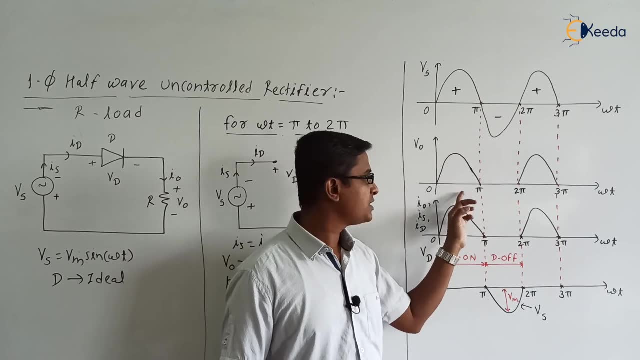 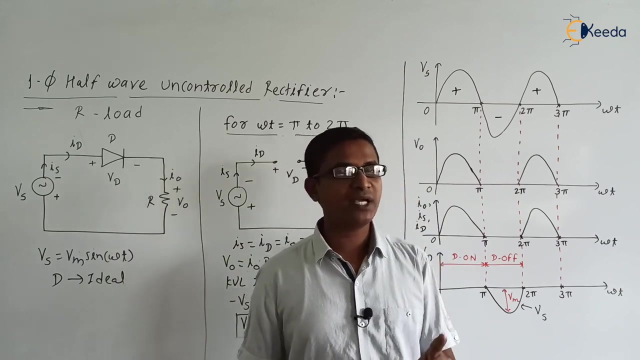 one input cycle. in the output we are getting only one pulse. that's why it is also known as single phase single pulse. single phase, single pulse. this is a single phase supply right and in the output we are getting only one pulse, so that's why it is also known as single phase. 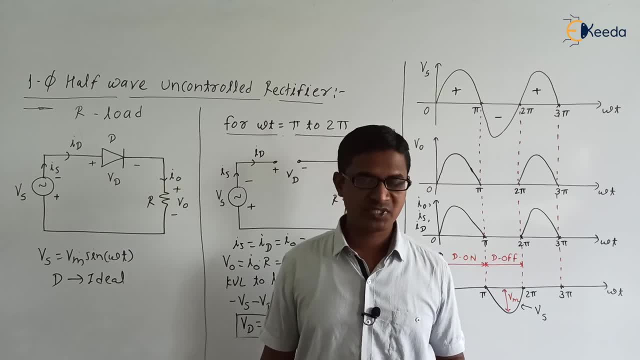 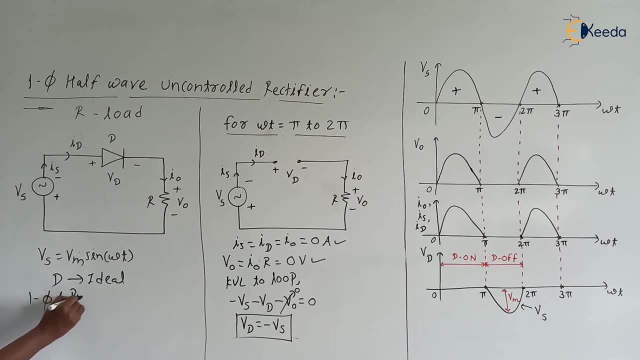 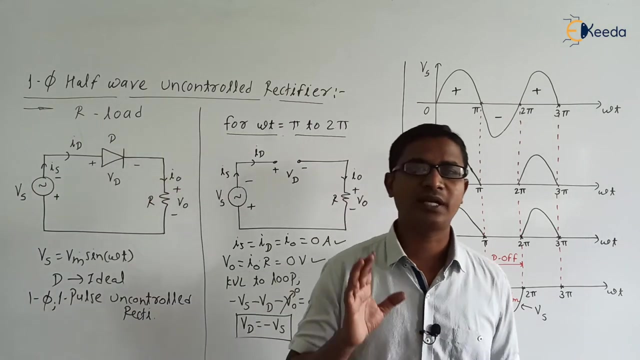 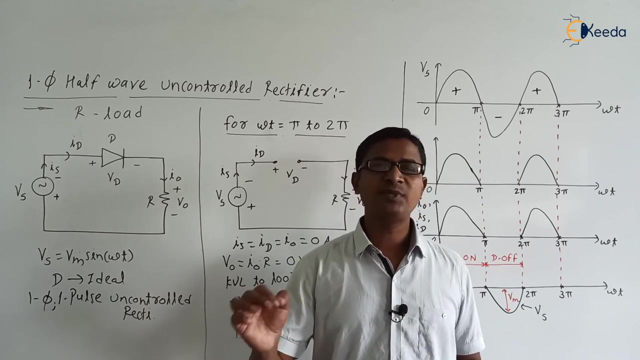 single pulse, uncontrolled rectifier. single phase single pulse, uncontrolled rectifier. i am writing here. some of the times they have used this word single phase, single pulse, right. single phase single pulse, uncontrolled rectifier. is this clear? are you getting the point, okay? so now my question is: if the input supply frequency is 50 hertz, okay, input supply. 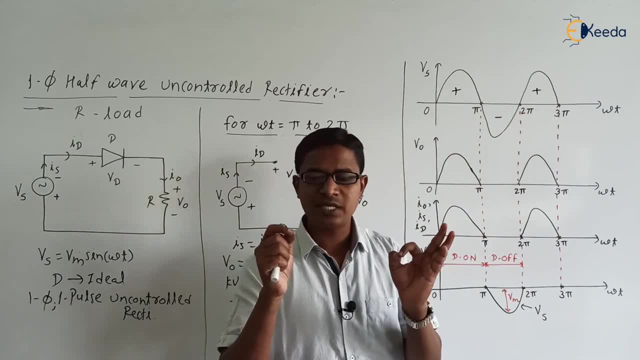 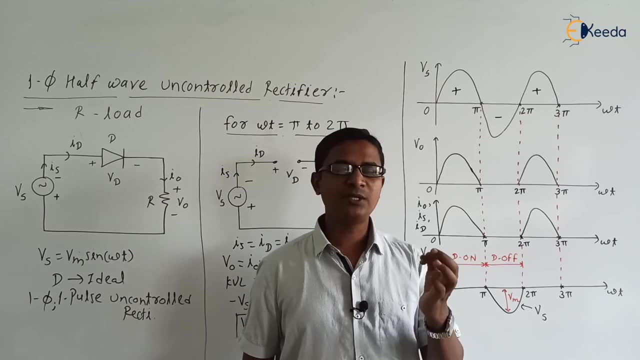 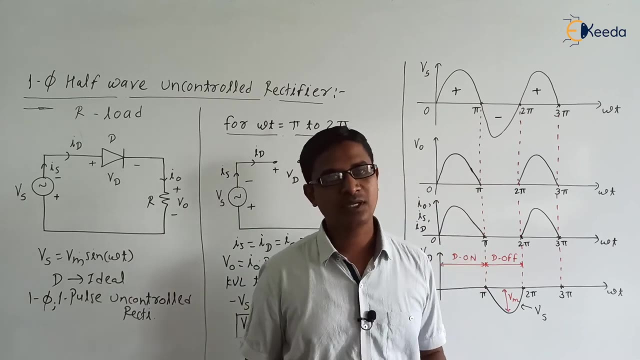 frequency is 50 hertz, the meaning is in the one second the input is completing 50 cycles. okay, frequency means what number of cycles per second? okay, if the input supply frequency is 50 hertz, then what will be the output pulse frequency, right, if you check, corresponding to one input. 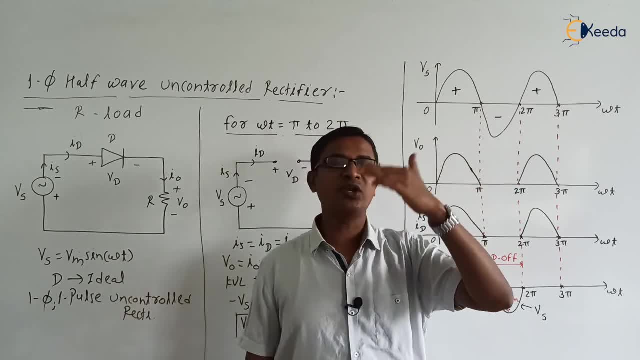 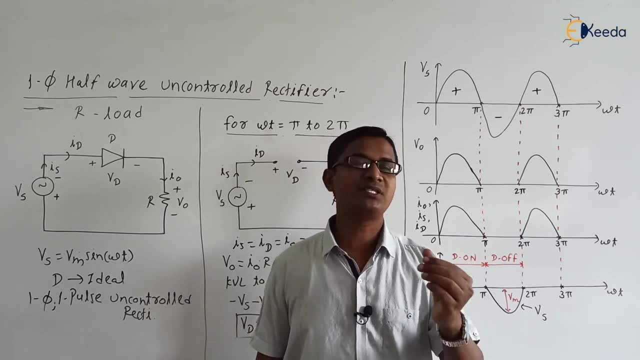 cycle in the output. we are getting only one pulse, so corresponding to 50 cycles in of the input in the output. how many pulses will be getting? will be getting 50 pulses only. are you getting the point, okay? so if the input supply frequency is 50 hertz,